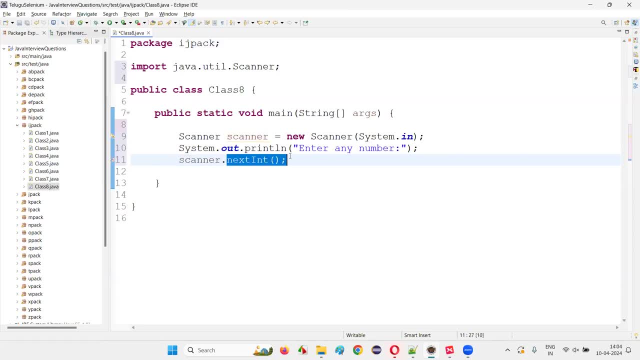 scanner dot. next int. that means we are expecting integer numbers. when I am watching this web site, We know that integer numbers are the Aygujun bride. We don't need to look for them because that's not affected. integer number from the user: okay, next int means we are expecting integer number from the user. 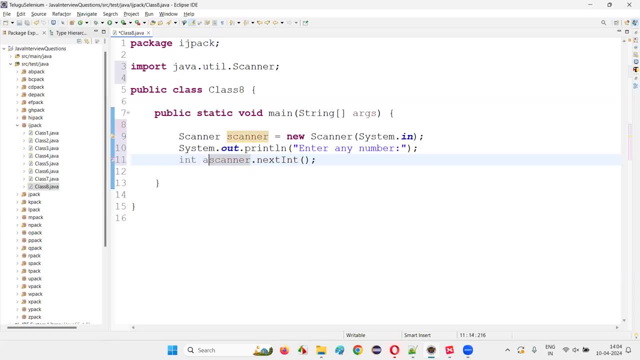 so that integer number i would like to store into a variable like int: a is equal to okay and systemoutprintln a. and at the end of this i'll write systemoutprintln- some sample statements. end of this program. like that, i'll write some sample statements here. end. 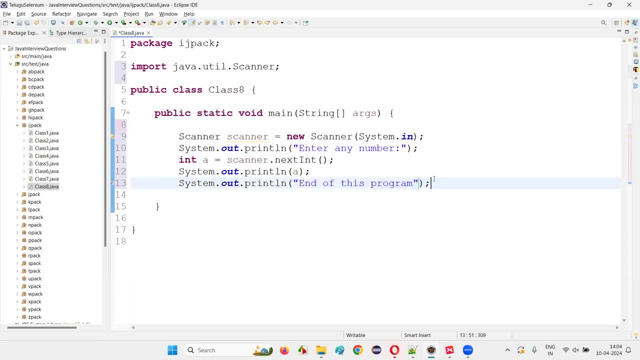 of this program like this. i'll copy paste this statement multiple times and just see here: one, two, three, four. now, after collecting the input, it is a good practice to close this scanner object, otherwise warning message will come. there's no error here, but you can close it at the best. 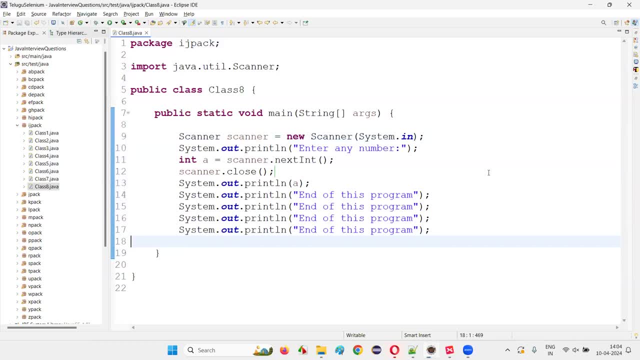 practice. now, if i run the code and if i really give a number, there is no problem with this. okay, the pro, when i run the program- the program is program- is asking the user to enter a number. if the user is entering a number, let's say nine, the same nine will be printed here and end of this. 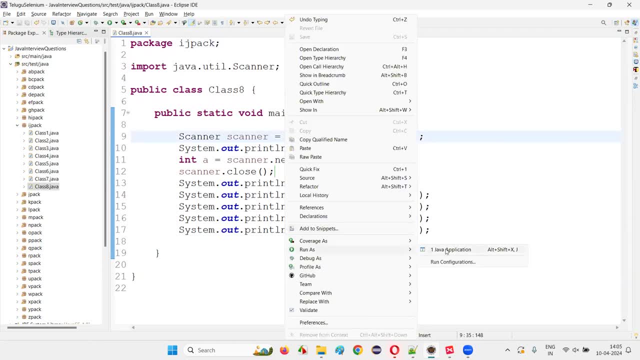 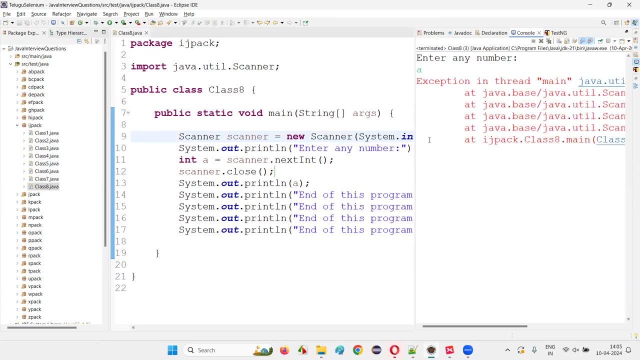 program will happen. the program will continue. what if the user, instead of giving a number here, next change is expected: integer number is expected instead of giving a number. if the user enters an alphabet presenter, immediately you are going to get an exception. that is, which type of exception you? 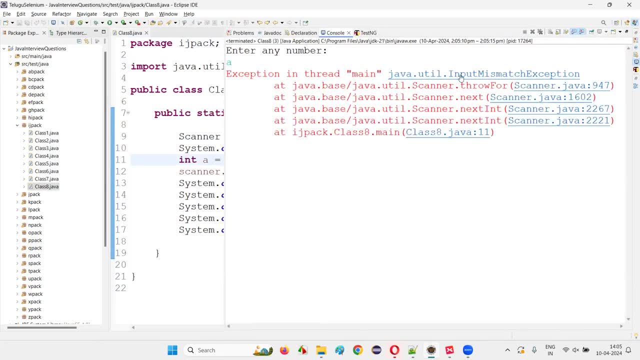 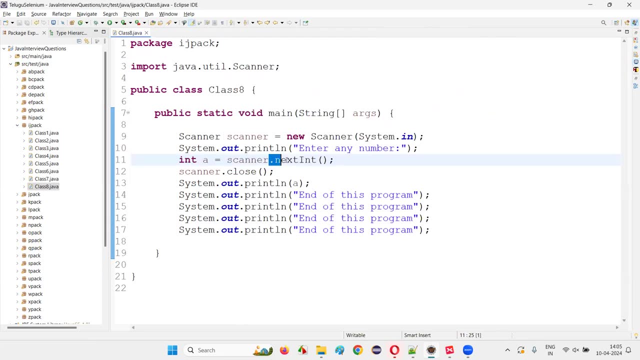 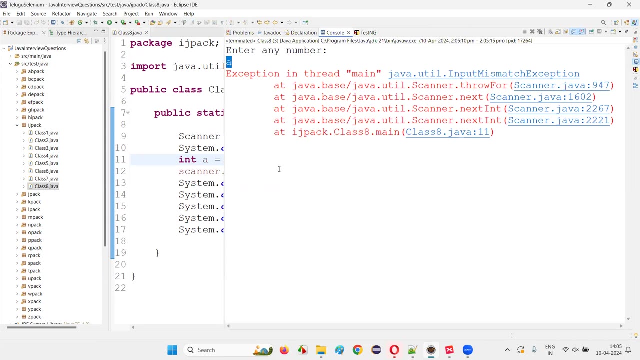 are getting here, guys, what type of exception you? you guys are getting here: input mismatch exception. the exception that i was talking about, that is input mismatch exception at the line level, because here input is required. but here you are passing as a user, you are entering alphabet, which is not a number right, it's not an integer number. so java immediately will give: 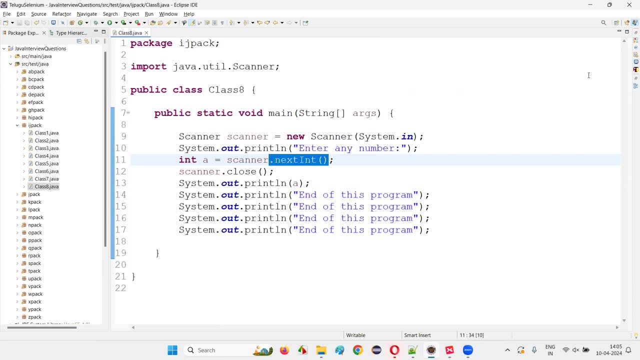 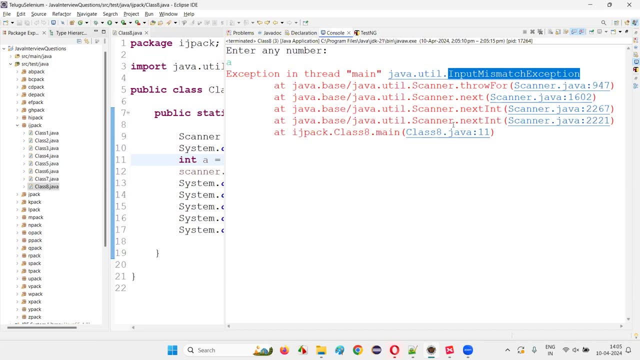 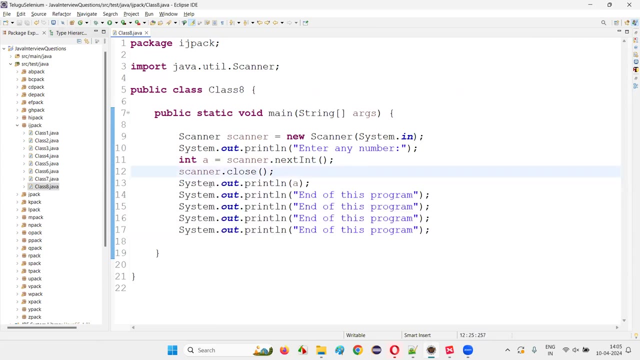 you. this next int command of java will immediately throw an exception from this predefined class, known as input mismatch exception. because of this exception or runtime error that occurs during the runtime, remaining parts of the program will not be executed. you see remaining statements after this particular exception has not been executed. even the scanner has not been closed here, because 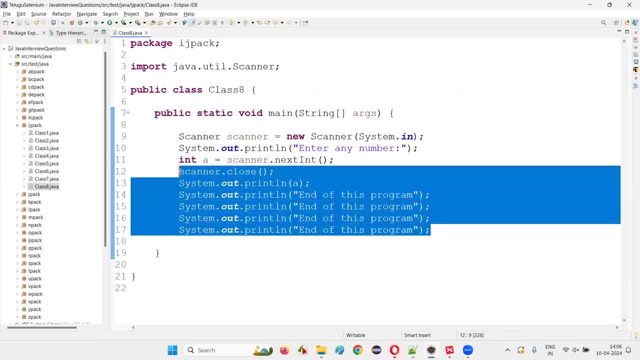 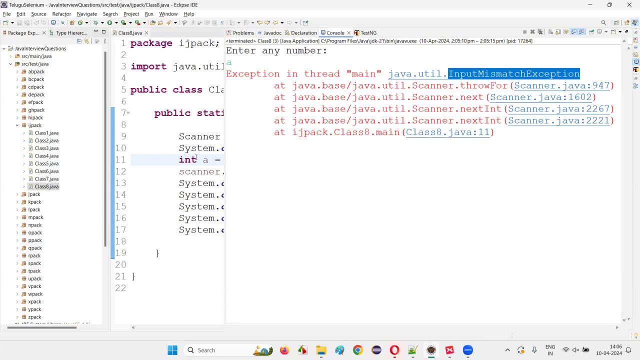 you got the exception here. so all these things, guys, okay, these statements have not gone, executed and uh, i've written and shown you a program where, which will result in an input mismatch. exception- where the program is expecting the user to enter during the runtime of this program, or